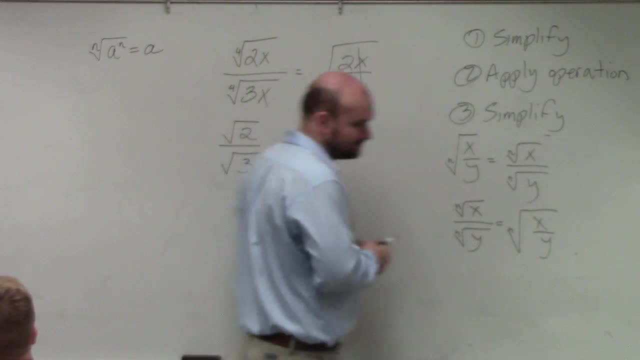 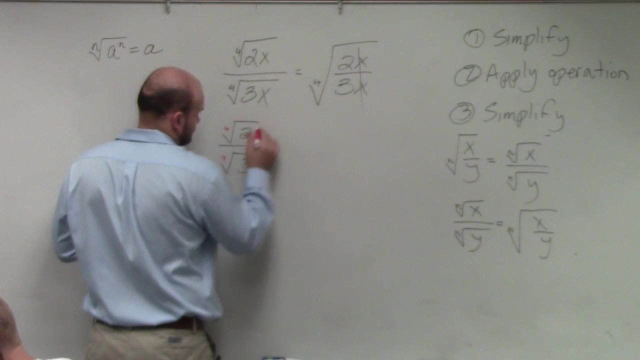 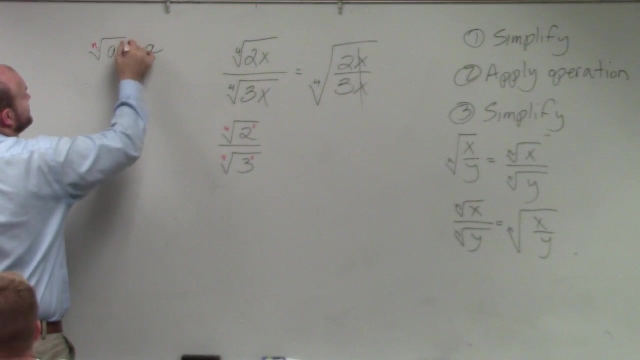 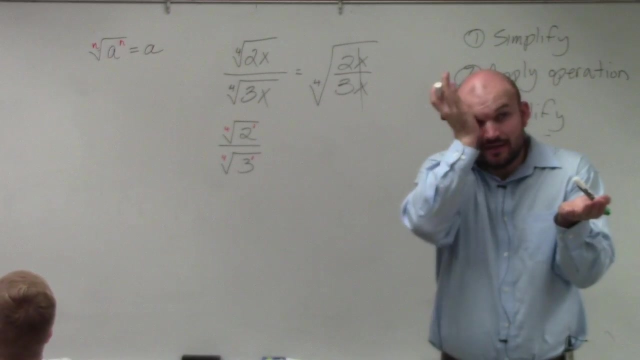 here. Let's put them in different colors. Maybe that will help you guys out. All right, So if everybody looks at this, Tyler, what I did is I rewrote the n in red, So you guys can really kind of see a difference with that. Now to be able to get the identity element, first of all, 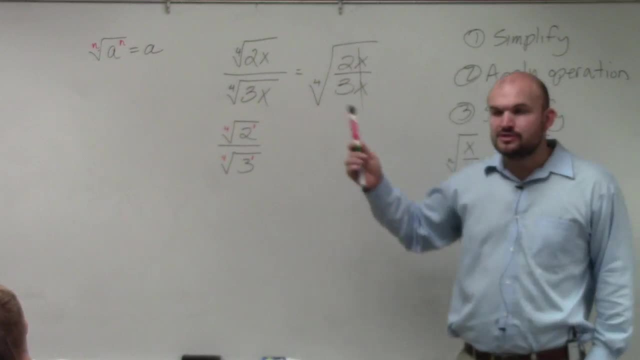 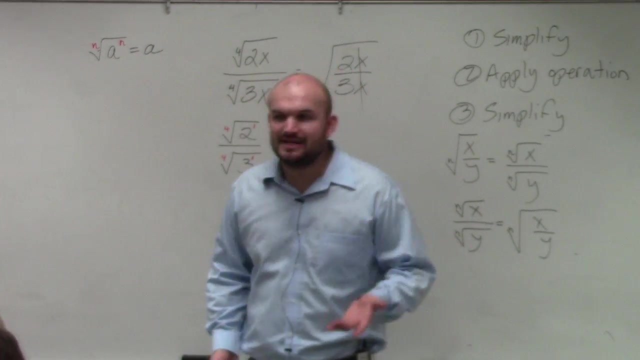 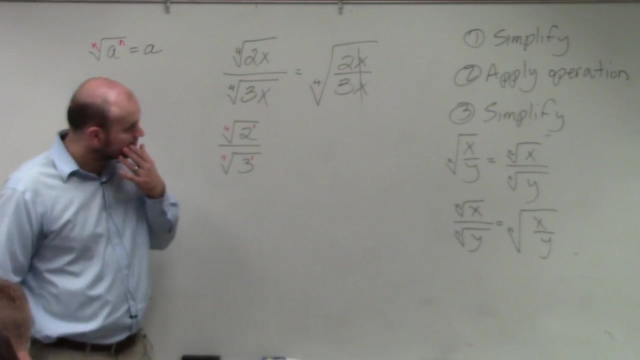 we understand that the three doesn't divide into two. So if you guys remember, when we were doing these problems with complex numbers, we didn't like dividing by complex numbers. Well, it's the same case with dividing by irrational numbers. We don't want to divide by irrational numbers. So since, since. 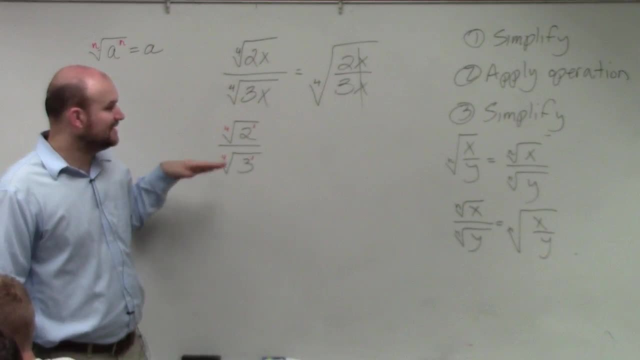 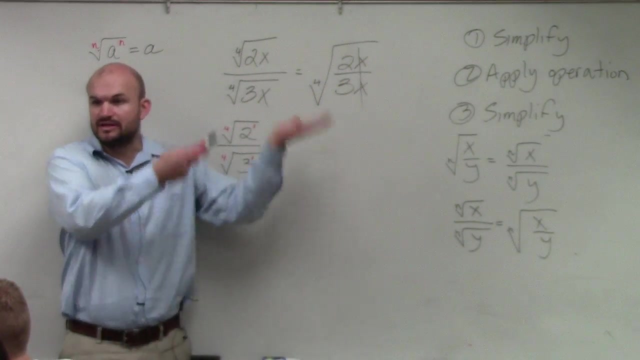 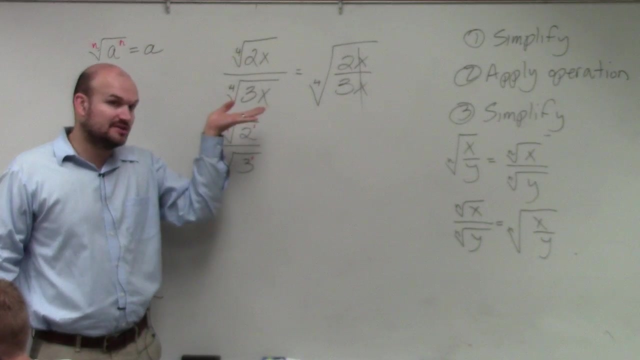 Eliza doesn't divide into it. what we can do is we can simplify it by removing the radical in the denominator. So the last problem: the number is divided into it. right And we're good. This problem: the denominator doesn't fully divide into the numerator, So we can't. 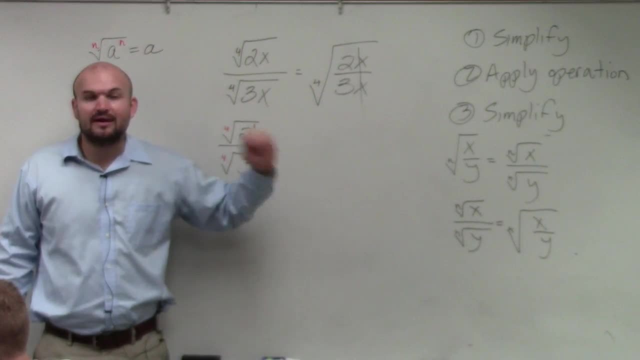 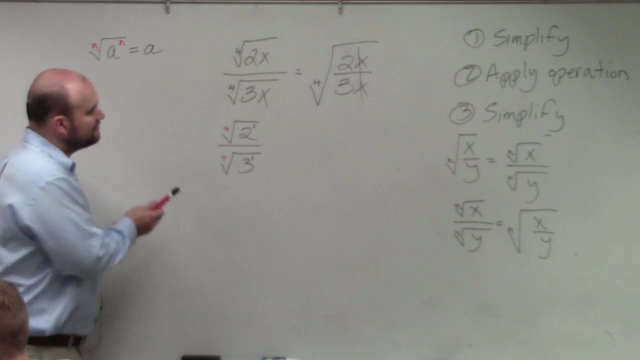 actually fully divide the problem, But what we can do is simplify it, And the way that we call it simplified is, if we can remove the denominator here, OK. So for this identity element to work, I have my three raised to a power of one. What power does my three need to be raised to for us to apply? 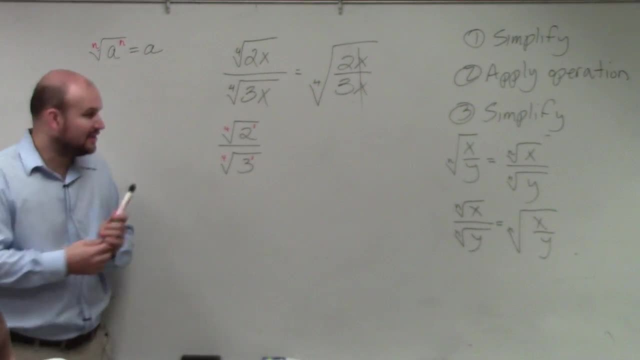 the identity element Four, Right. So therefore, what do I need to multiply three to the first power to to get three to the fourth, Which would be Keith? What would it be Three to what power would give me? do I need to multiply this by? 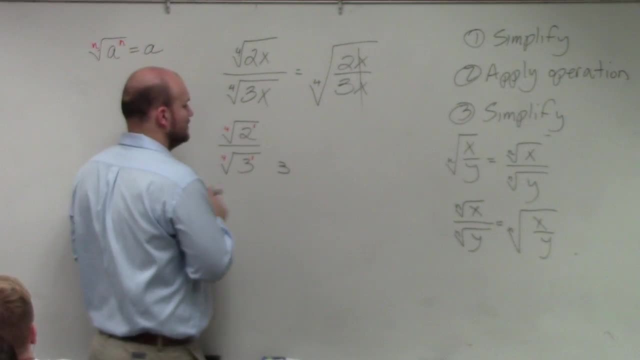 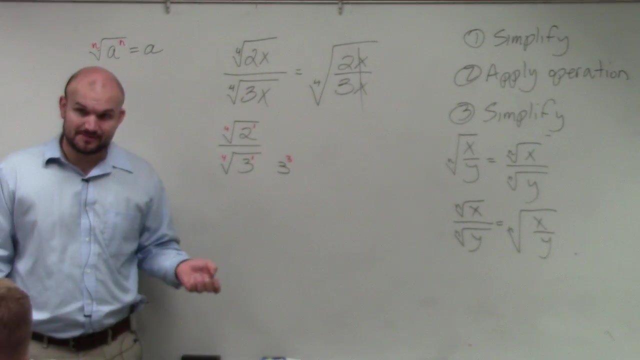 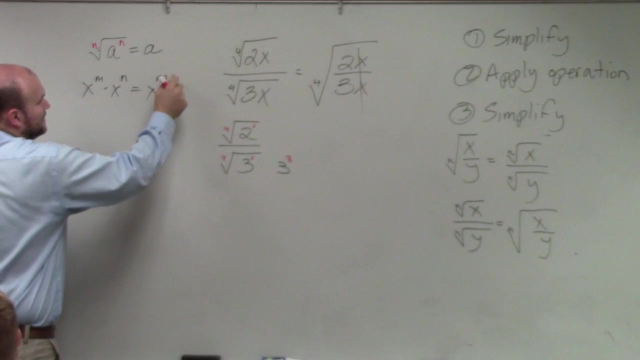 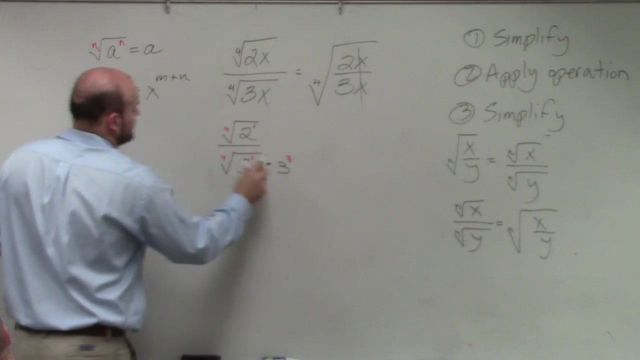 Three cubed. Remember last class period we did the rules of exponents. If you have x to the m times x to the n, that equals x to the m plus n. Three to the first power. times three to the third power equals three to the fourth power. 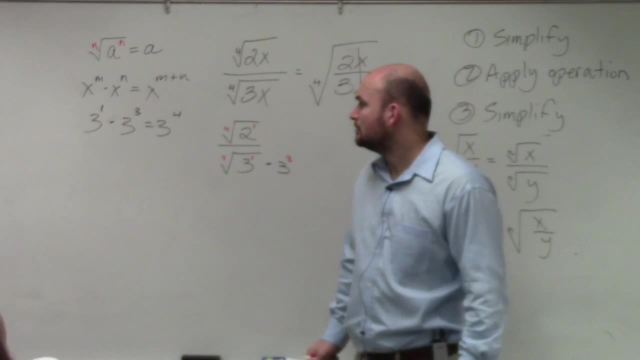 Why aren't you multiplying the three? Because that's not what the rule of exponents says. X to the m times x to the n equals x to the m plus n. Three to the first power times three to the third power equals three to the fourth power. 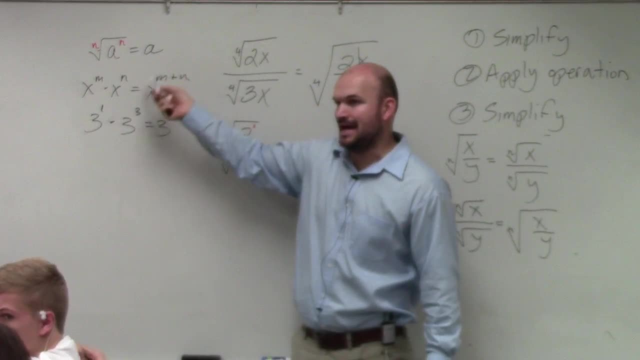 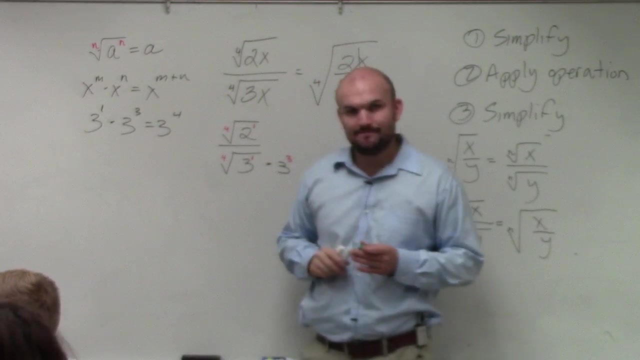 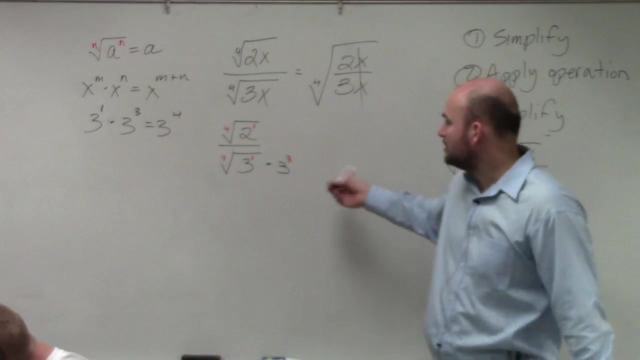 x to the m times x to the n equals x to the m plus n. 3 to the first times 3 cubed equals 3 to the fourth. OK, That's basically the rules. The only difference with the rules is, instead of x's, you're having some variables. 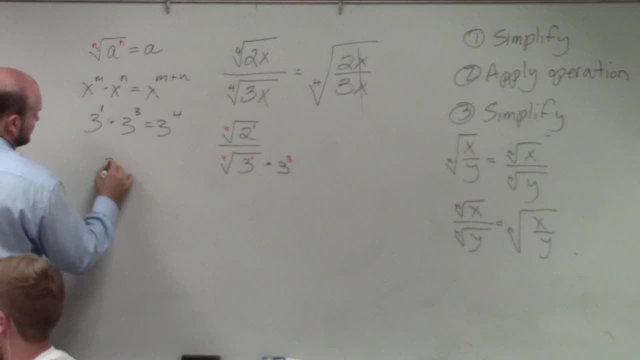 Now, here comes the problem, though, with looking at this. Yeah, I'll get to that in a second. Here comes the problem. Can you do 3 times the square root of 3?? Does that equal the square root of 9?? 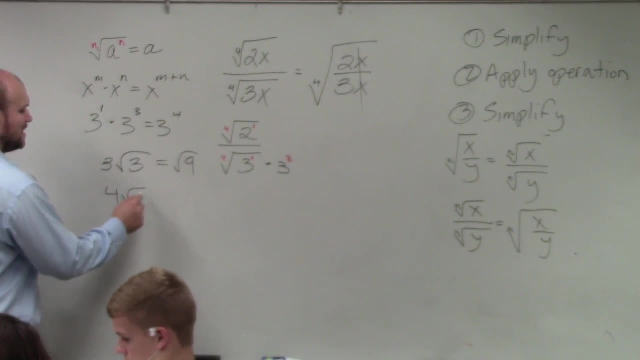 No, it doesn't. And if you guys don't believe me, do this: 4 times square root of 4, that does not equal the square root of 16.. Right, Because what's the square root of 4? 2.. 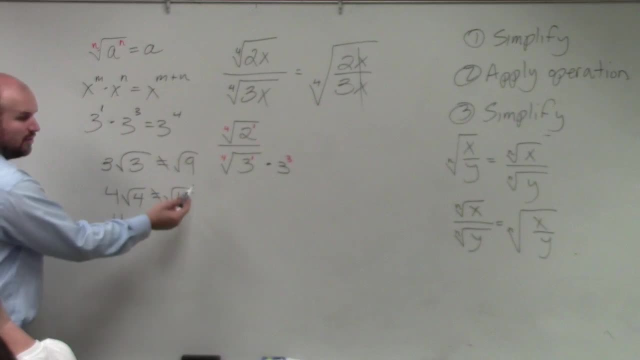 4 times 4.. 2 equals 8.. Right, The square root of 16 is equal to 4.. So do you guys see how that doesn't work? So, Kelsey, the main important thing, to be able to multiply this what we have to do. 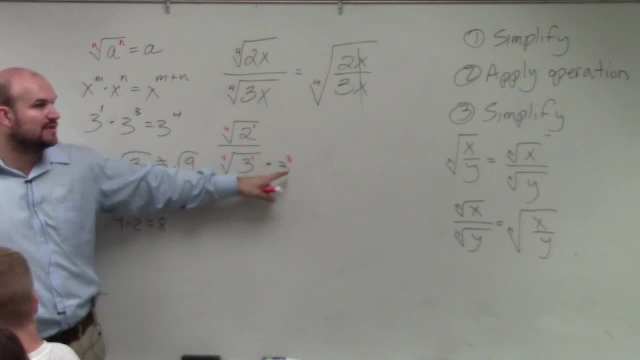 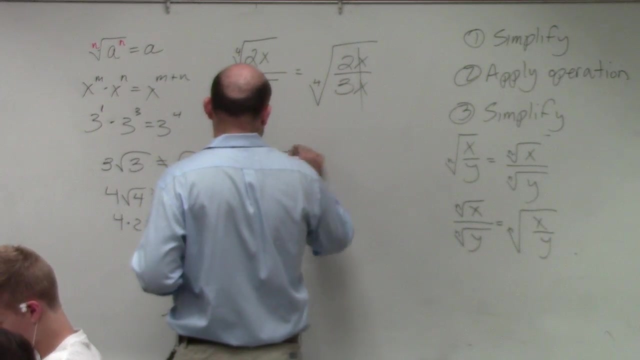 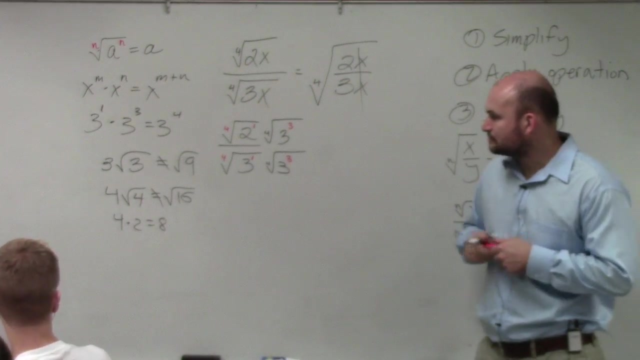 is, we have to have this under a root And we have to have it under the fourth root. So, to finish this problem, to rationalize the denominator, what we simply need to do is multiply this. So what we're going to do is we're going to multiply this. 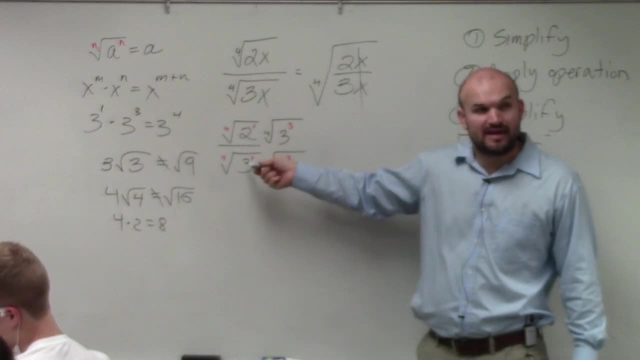 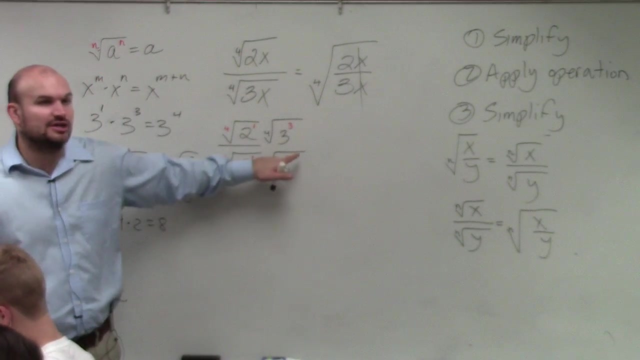 by the same root And again I got this value because this is what's going to make my identity element in the denominator. Usually I don't like to actually tell you or figure out what the number is. We know 3 cubed is what? 27?? 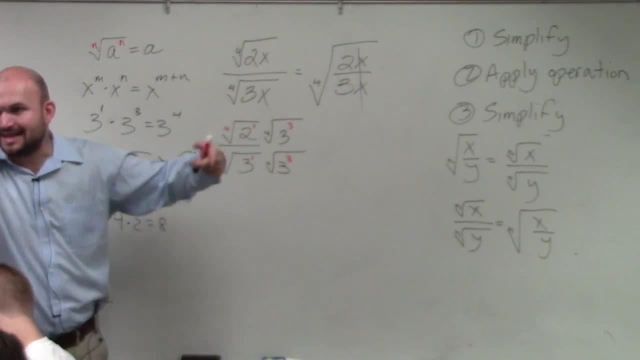 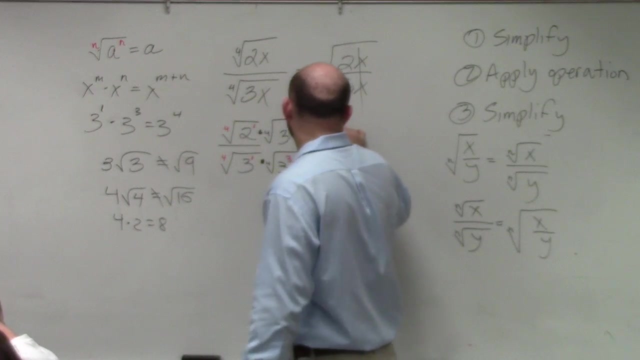 Right. Rather than writing it as 27,, I like to keep it like this Again, so you can see, using the rules of exponents. So when I multiply this across, I have the fourth root of 2.. Now here I'll simplify it: times 27,. 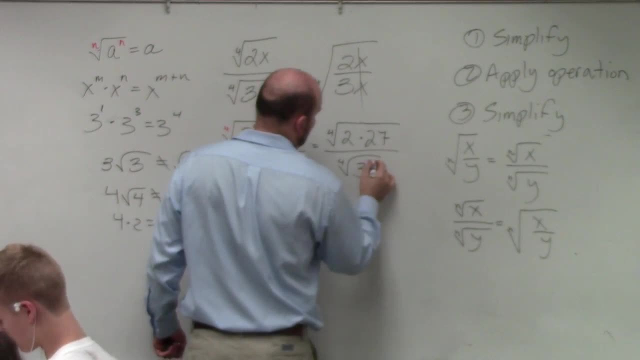 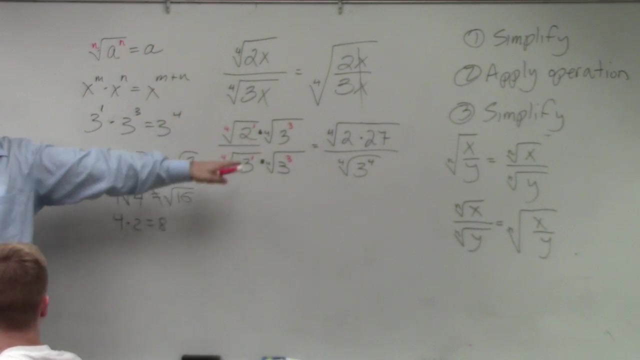 all over the fourth root of 3 to the fourth power. So now we have the fourth root of 3 to the fourth power. Do you guys see how now I can get rid of my root? Because what's the fourth root of 3 to the fourth power?